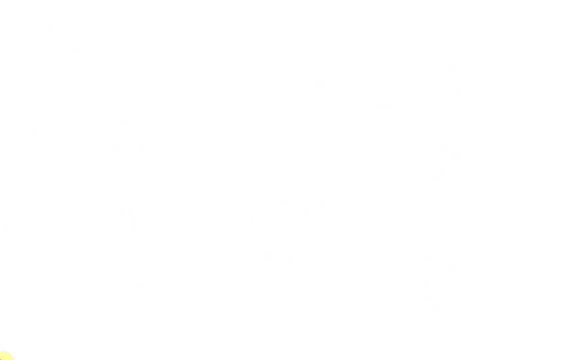 next generation firewalls. so what are the packet filters? so we have already discussed that the traffic or the data on the internet travels in packets and, as the name suggests, that the packet filter firewalls check the authenticity of the packet. if the packet is right, then it would allow it to pass, and if it, 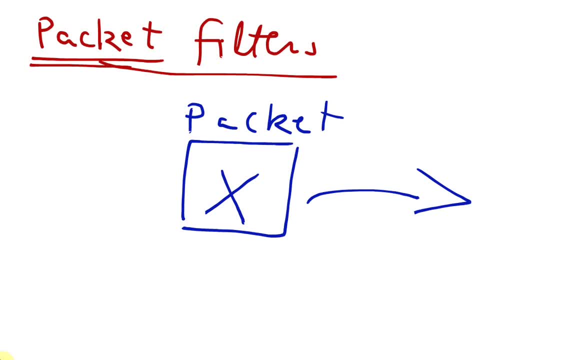 is malicious or malicious or malicious, or if it's harmful, then it will not allow that packet to be passed. so let's discuss in detail about packet filters, firewalls. so, as I have already told you that a firewall is a computer or is a software or hardware security system. 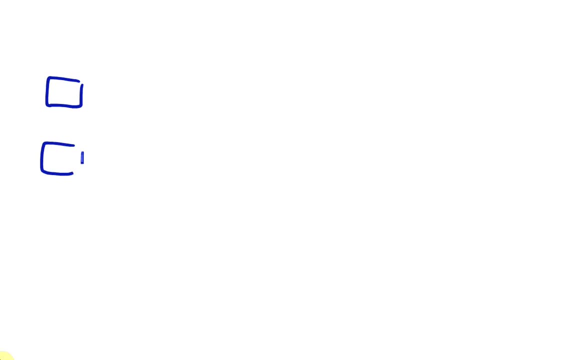 which sits between your internal network- that may be your home network or the office network- and the external network, and in most cases, this internal, external network is the internet. so we have got an internal network and we have got an external network, and a firewall may be a software that is installed on a 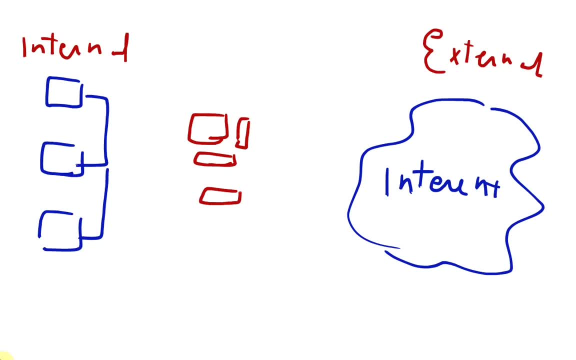 server. it can be a hardware firewall, or it can be installed in a router, or it can even be a proxy server, so we can install these packet filters firewall in different companies, depending on our requirements. so let's suppose that a packet will have a network that is offering specific棒 user right from the device to, or anyway an Windows server will be able to install a packet. Yay, ready. well, let's switch back to the screen. 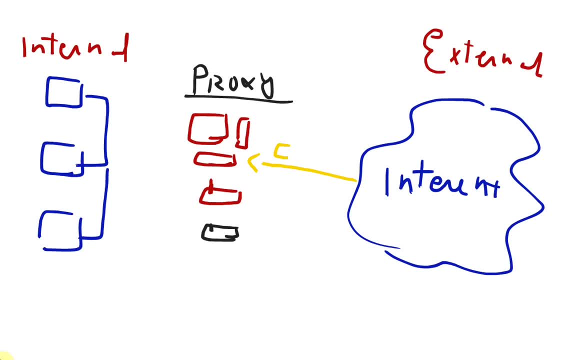 reaches to our firewall, that is, the packet filter firewall, from the internet, then the firewall is acting as an inspector that it inspects that packet. that is, it inspects the packet source address, because every packet has got a source address it checks it will. 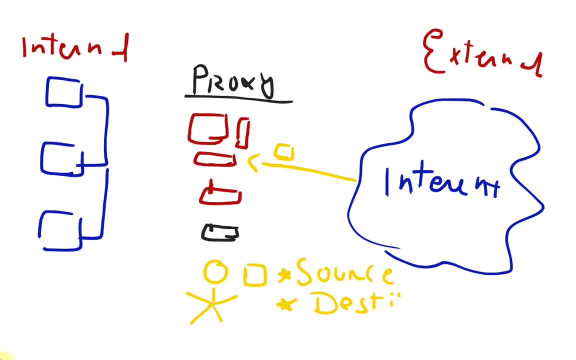 check its destination address and it will check its protocol. there are different protocols on the computer networks and if we have disabled any of the protocol then it will not allow that packet. So these packet filters, these firewalls, will check if the packet has got the source address and if it has got. 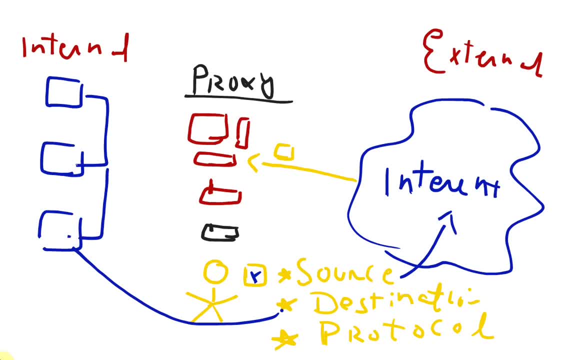 the destination address and if the destination address is the part of our network and if the packet is to be delivered to a port, that is, if we have allowed that port to be able to, to be able to receive those packages, packets. so there are a thousand of thousands of ports. 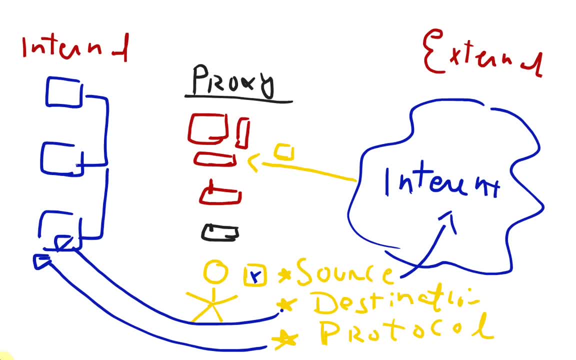 on our computers and if those protocols, and if that protocol or that port is allowed, then the firewall would allow the packet to be delivered to our internal network and vice versa, if the packet is delivered to an external PC, then the firewall would check. 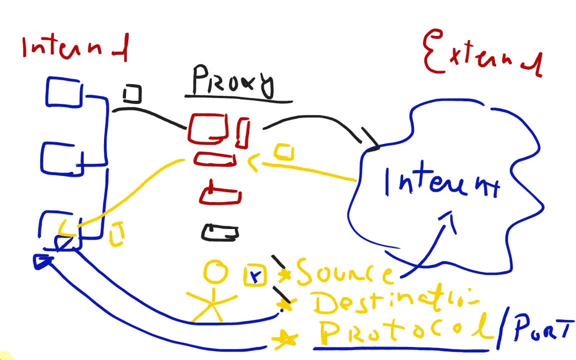 if it has got the source address, if it has the destination address and if the protocol is allowed to be able to deliver to the internet. For example, let's suppose if we have blocked our firewall, FTP or Telnet ports, then those would not be able to pass. 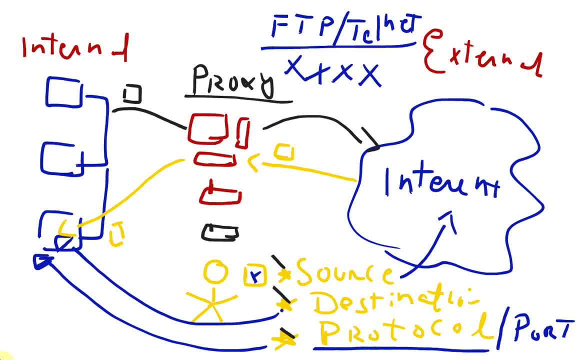 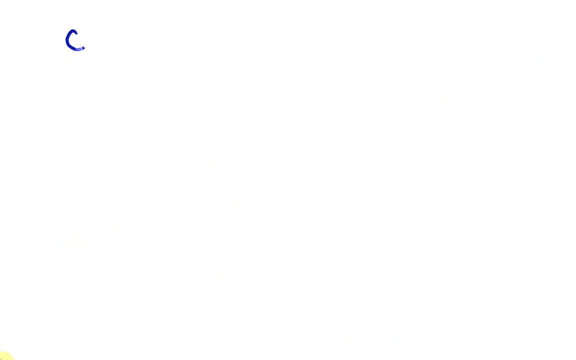 So this is how a packet filter's firewall operates and packet filter firewalls operates on the first three layers of OSI model. we have already discussed about OSI model in our previous tutorials, So if you are not familiar with the different layers of seven layers of OSI model, then 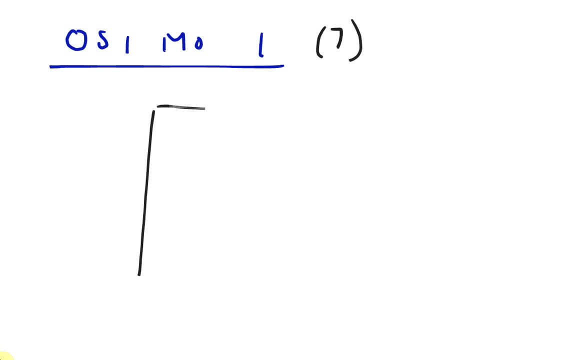 please visit my previous tutorials. So we know that at the bottom the first layer in OSI layer or layer model is called the physical layer. and then we have got the physical layer, and then we have got the physical layer, Data link layer and on number three we have got network layer. 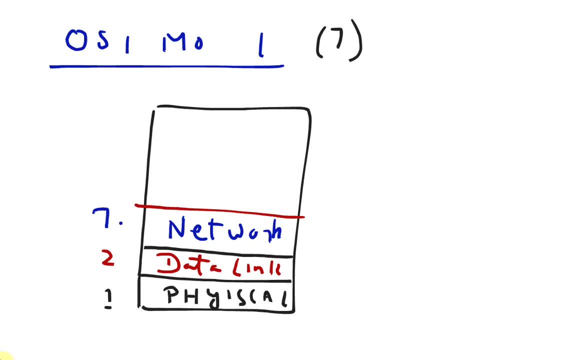 So these packet filter firewalls operated and are still operate on these three layers of OSI model and these packet filter's firewalls are called stateless layers. They are called stateless firewalls because they do not check or cannot check the session or the connection status of the communication. 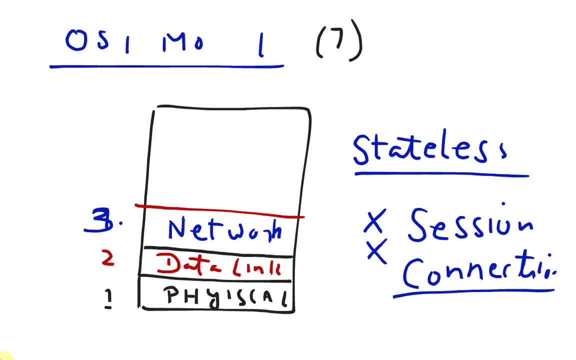 So these are called the stateless firewall. So they only check the packets and, for example, in TCP, most of the packets on the internet which are delivered in TCP or to UDP and these so most of the traffic on the internet. 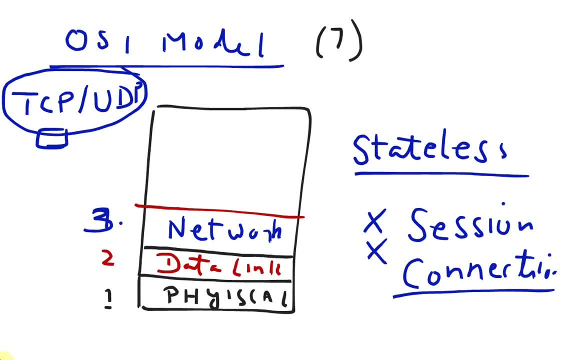 is being delivered with the help of the TCP IP protocol protocols or UDP protocols. So these firewalls can only check the TCP status of the packet and it would allow the packet if that TCP has some address or if the UDP has the destination address. 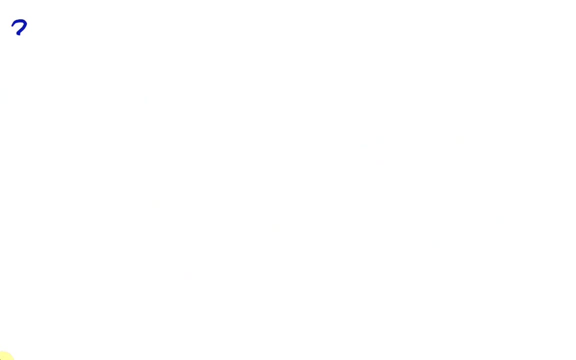 And the second generation of the firewalls are called stateful firewalls. They act as the packet filters, but in addition to the packet filters they have the capability to check if the session has already been established or if that packet is intended for a new session. 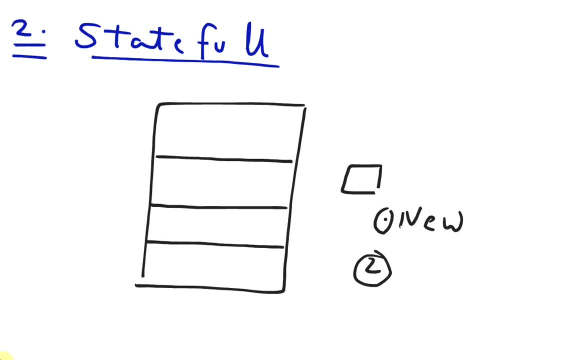 or if that packet is intended for an existing session or the existing communication that is being done between the host and the source computer, or if that packet is not a part of any communication. So if it's not a part of any communication, then it could mean that it's a malicious packet. 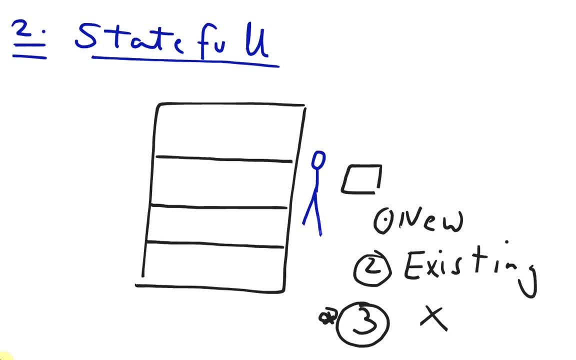 and the inspector within the firewall would check it more rigorously. So these stateful firewalls, in addition to physical data, link network layers. it also operates on that. The third one is the transport layer and based because it can operate on the transport. 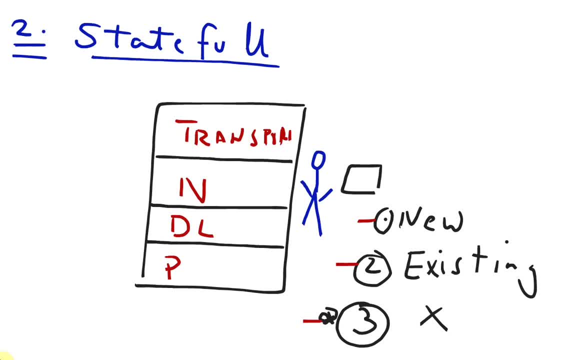 layer. it can check the status of the session or connection, Because we have already discussed that TCP is a connection-less protocol and IP operates roughly on the transport layer of OSI And IP is a stateful protocol, So it can check the status of the connection. 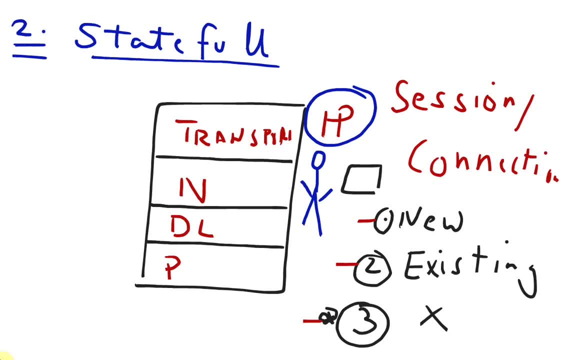 And as these stateful packet filters or stateful firewalls can check the status of IP addresses, therefore they can check if the session is already established, if it's a new session or if that packet is not a part of any communication And, based on the predefined set of rules, it would either allow the packet or it would. 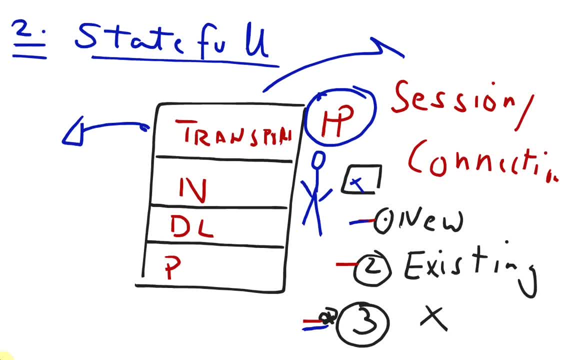 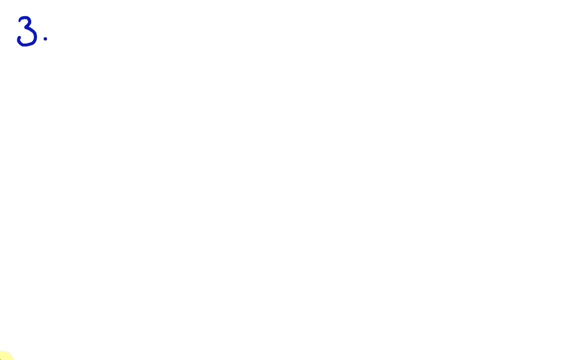 deny the access of that packet to our internal network and send that, drop that packet and send an error report to the sender. And the third generation of the firewalls. in addition to packet filtering and stateful firewalls, they also act as an application layer. 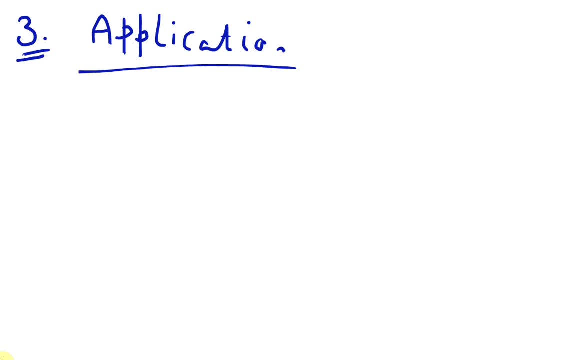 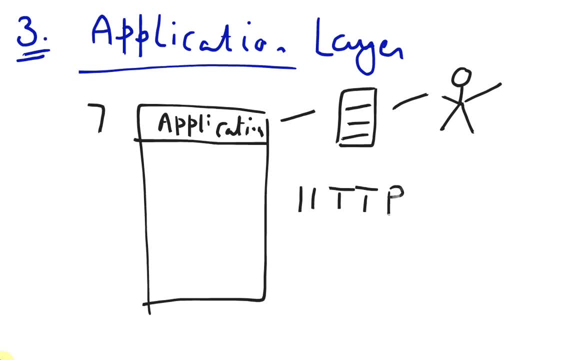 And some of the protocols, For example, HTTP protocol that is being used for the web communication, FTP protocol or DNS services. They are the high level protocols and they act at the application layer And these firewalls can allow the traffic based on those protocols. 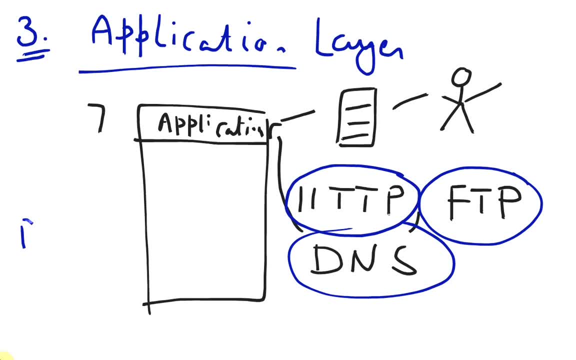 So packet: Application layer protocol. Packet Application layer protocol. Application layer protocol. Baggie function of network Banner Task Manager. Most of the firewalls can check for the ports, if those ports are open or not And if those packets are using some special protocols. 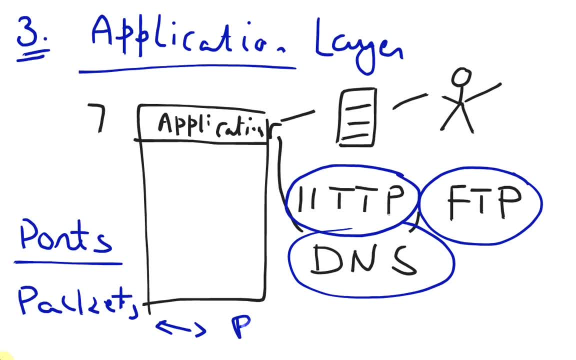 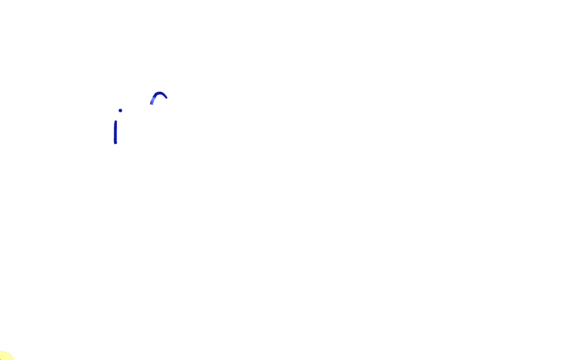 So, for example, if on our network we have not allowed the communication through FTP protocol, file transfer protocol, then all the packets using those protocols would be denied. Thank you for watching this video. So, guys and girls, thank you very much for joining me in the second tutorial on firewalls. 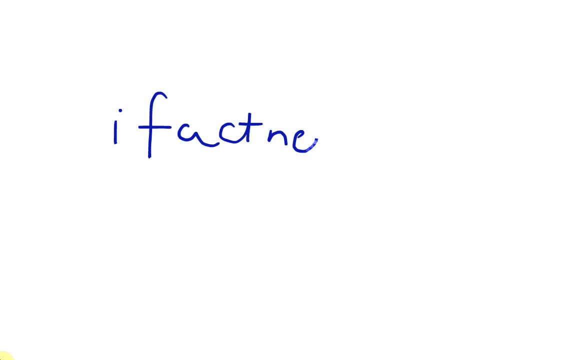 If you would like to know more, then please visit ifactnercom. In the next tutorial, we would be discussing about different types of firewalls that are available in the market. So see you in the next tutorial, Take care, Bye.